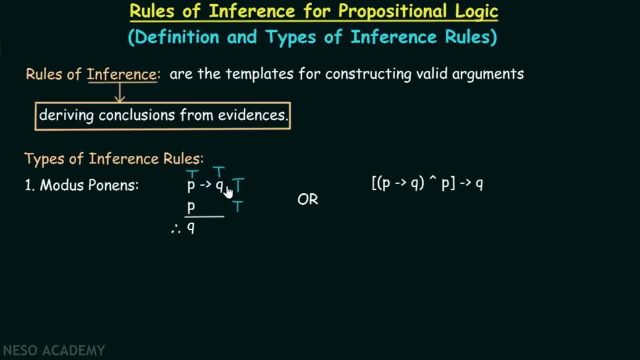 then Q has to be true. It cannot be false. Therefore, conclusion must also be true. Right, This is the law of modus ponens. We can also write this argument as: P implies Q and P implies Q. We know that. these are the premises. 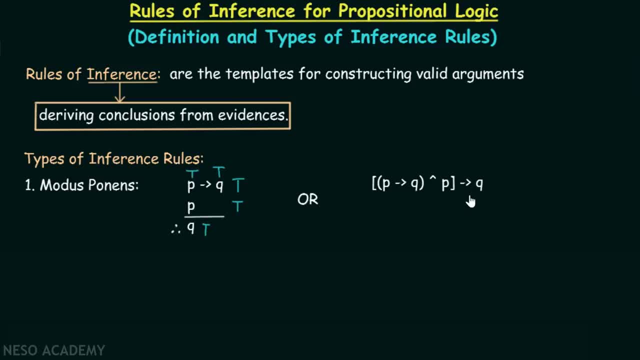 That is P, implies Q And P, And this is our conclusion, that is Q, And we know that premises always implies conclusion Right, And hence we can write this argument in this form. Okay, now the second rule in this list is modus ponens rule. 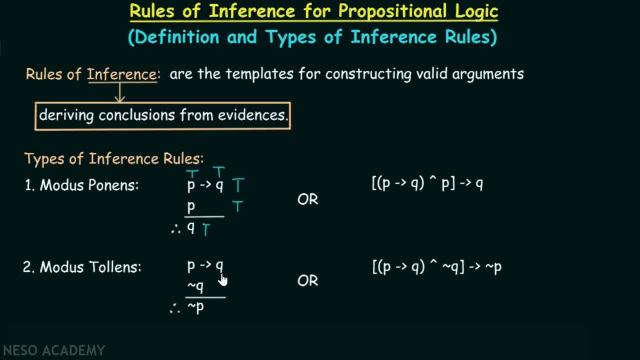 According to this rule, P implies Q, not Q, therefore not P. Now, as we know, P implies Q is true and not Q is true. Therefore, we need to conclude that not P is also true. Therefore, we need to conclude that not P is also true. 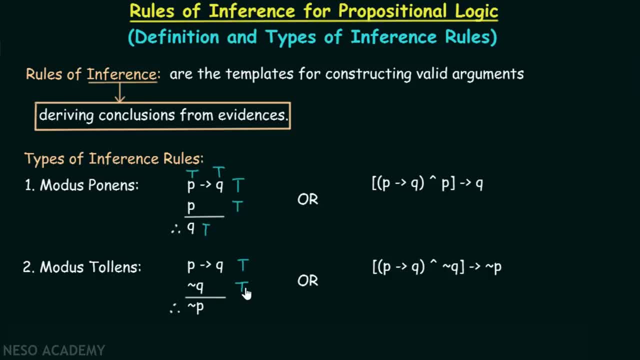 Therefore we need to conclude that not P is also true. Now, if P implies Q is true and not Q is true, then Q becomes false Right Now. if Q is false, then P has to be false. It is not the case that P becomes true. 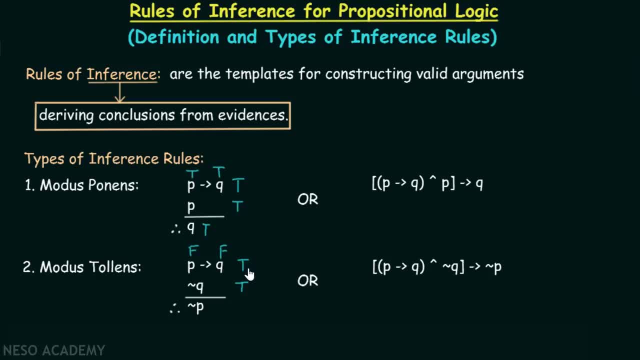 Because if P is true, then true implies false is false Right Now. if P is false, then not P will be true. Therefore, we can say that our final conclusion becomes true And hence this argument is a valid argument. Definitely, we can write this argument. 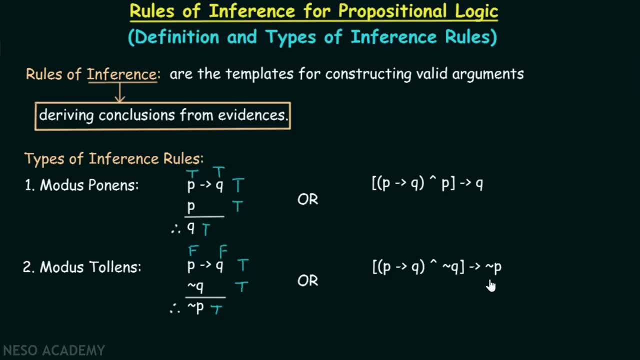 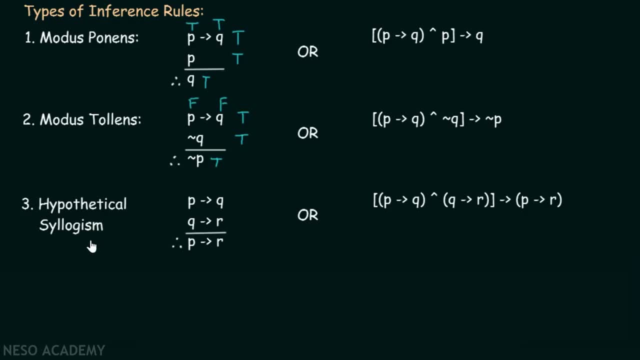 as P implies Q and not Q implies not P, Right? Let's consider the third rule in this list, that is, hypothetical syllogism. According to this rule, P implies Q, Q implies R. therefore P implies R. Now, if P implies Q is true and Q implies R is true, 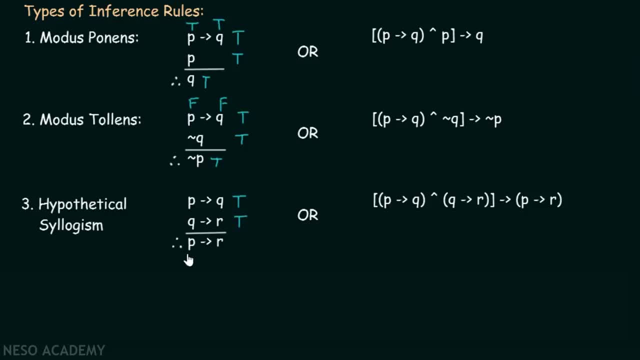 then P implies R has to be true. Let's try to make this P implies R false by taking P true and R false. Let's see whether we would be able to make it false or not. Let's take P true and R false. 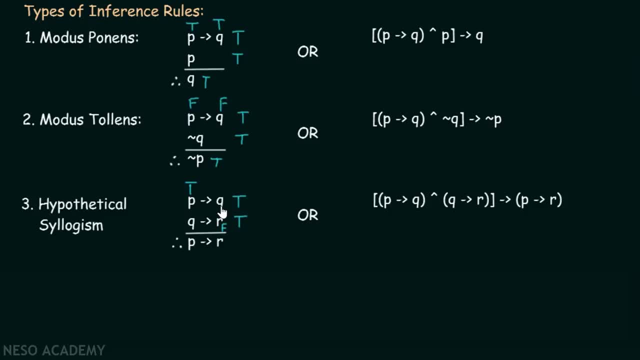 Now, if P is true, then Q cannot be false Right. Q has to be true, And because Q is true, then R cannot be false Right. Therefore, R has to be true. It cannot be false Hence this has to be true. 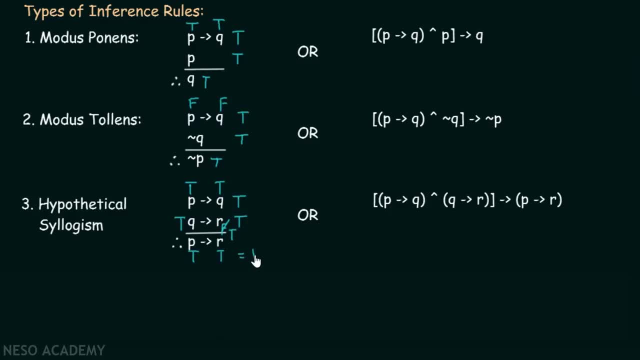 And if R is true and P is true, then true implies true is always true. Therefore, we cannot make P implies R false And definitely we can write this argument as P implies Q and Q implies R implies P implies R. Let's consider the fourth rule. 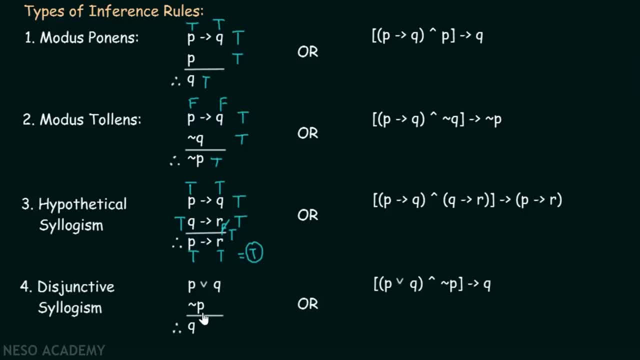 that is disjunctive syllogism: P or Q, not P, therefore Q. Now let's say P or Q is true and not P is also true. If not P is true, then P becomes false, And if P is false, then Q has to be true. 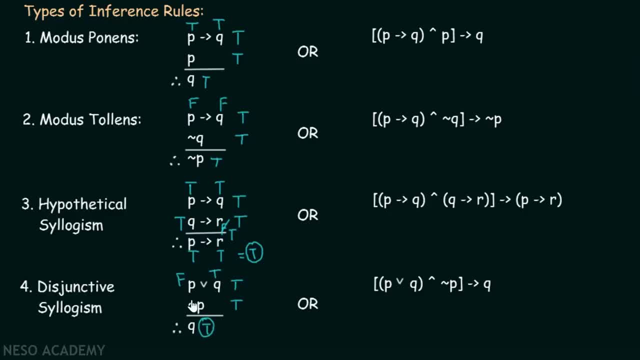 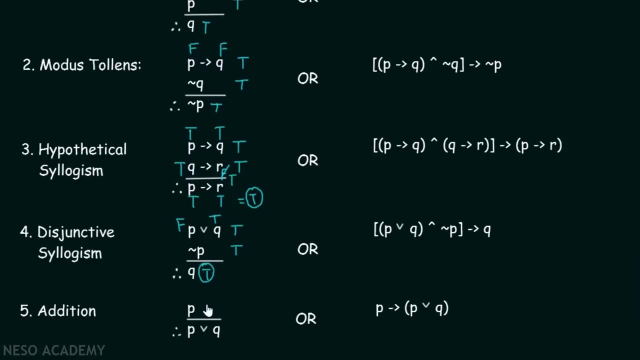 Therefore, finally, the conclusion becomes true And we can write this argument as P or Q, and not P implies Q. Now let's consider the fifth rule, that is, addition rule P, therefore P or Q, How this argument is valid When P is true. 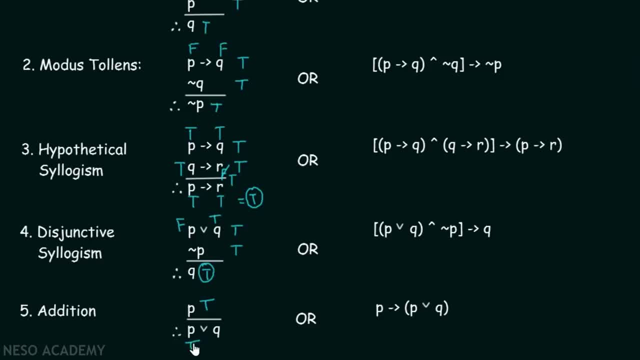 then definitely this is also true. If this is true, then true, or with anything is always true, Then the argument is always satisfied, Right. Hence we can say that this argument is valid And we can write this argument as P implies P or Q. 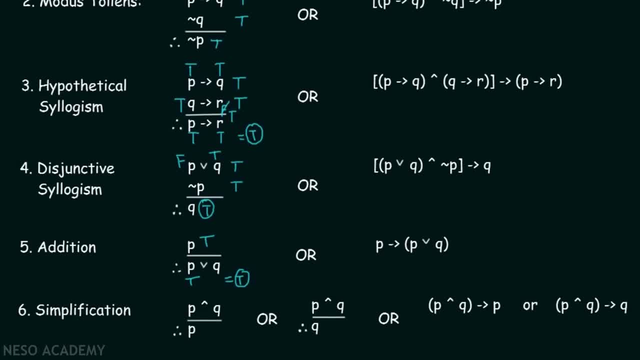 Let's consider the sixth rule, that is, simplification rule. P and Q therefore P, or P and Q therefore Q, Or we can write these arguments as P and Q implies P, or P and Q implies Q. Right Now why these arguments are valid. 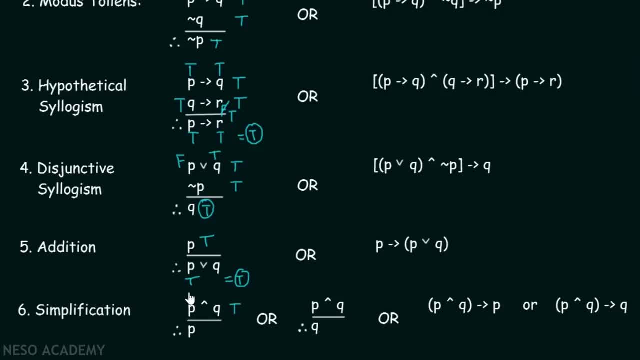 As P and Q is true. this can be true only when P is true and Q is true. Therefore, we can say that both P is true and Q is also true, And hence both the conclusions are correct. Hence we can say that these arguments are valid arguments. 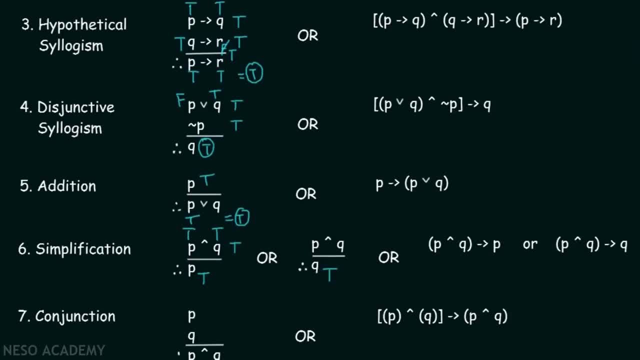 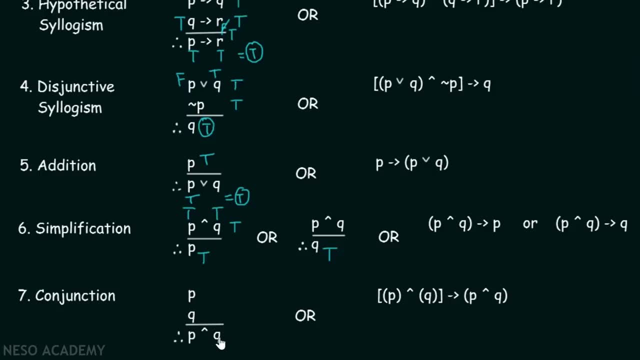 Right, Let's consider the seventh rule, that is, conjunction rule. P, Q, therefore P and Q. Now, if P is true and Q is true, then definitely P and Q becomes true, Right? This is according to the conjunction law.